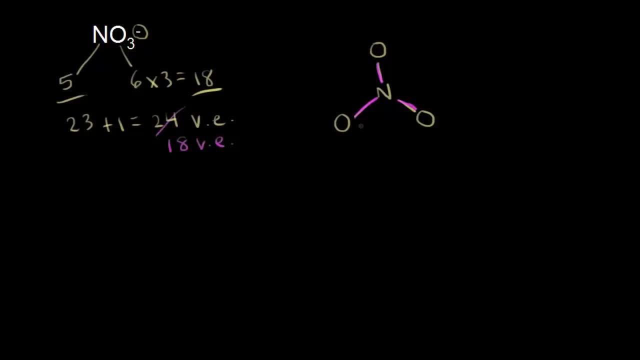 And oxygen is going to follow the octet rule. Currently, each oxygen has 2 valence electrons around it, The ones in magenta. So if each oxygen has 2, each oxygen needs 6 more to complete the octet, And so I go ahead and put 6 more. 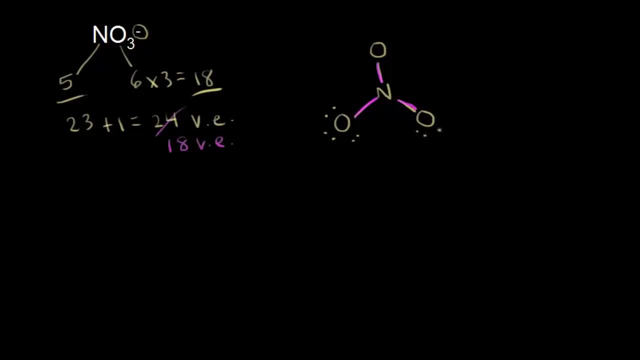 And put 6 more valence electrons on each one of my oxygens. Now each oxygen is surrounded by 8 electrons, So the oxygens are happy. We added a total of 6 valence electrons to 3 oxygens, So 6 times 3 is 18.. 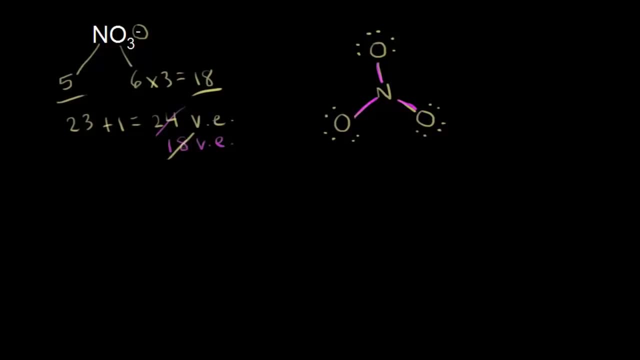 So we've used up all of the electrons that we need to represent And so this dot structure so far it has all of our valence electrons. here. Oxygen has an octet, so oxygen is happy, But nitrogen does not have an octet. 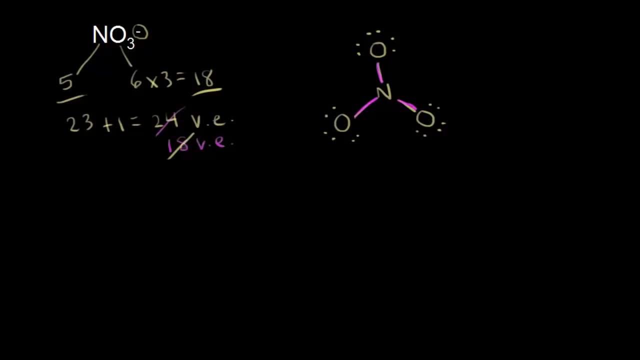 If you look at the electrons in magenta, there are only 6 electrons around the nitrogen, And so the nitrogen wants to get to an octet. And there are a couple of different ways that we could give nitrogen an octet. For example, we could take a lone pair of electrons from this top oxygen here. 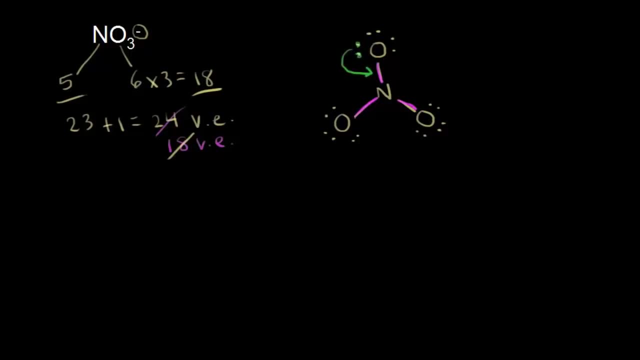 And move them into here to share those electrons between that top oxygen and that nitrogen. So let's go ahead and draw the resulting dot structure So we would have our nitrogen now with a double bond to our top oxygen. Our top oxygen had 3 lone pairs of electrons. 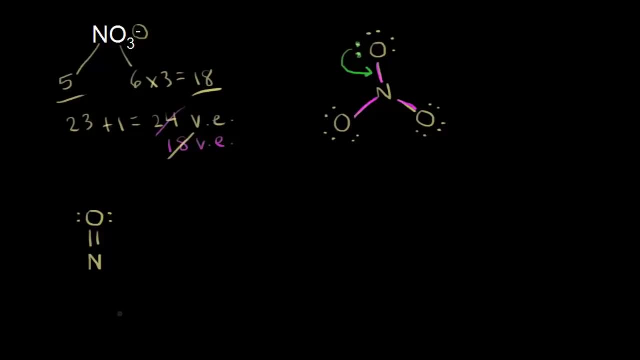 But now it has only 2 because the electrons in green moved in to form a double bond. This nitrogen is bonded to an oxygen on the left here, on the bottom left, And an oxygen on the bottom right here. So this is a valid dot structure, right? 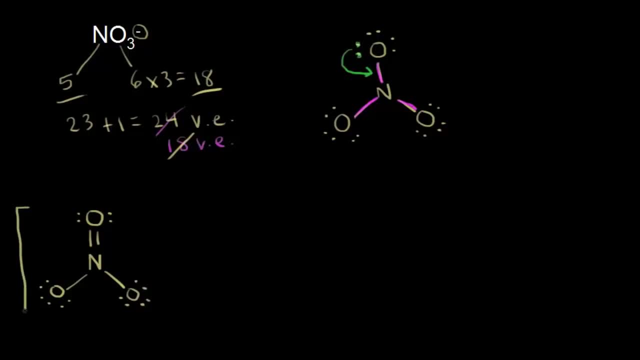 We followed our steps And we'll go ahead and put this in brackets And put a negative charge outside of our brackets like that. So that's one possible dot structure, But we didn't have to take a lone pair of electrons From the top oxygen. 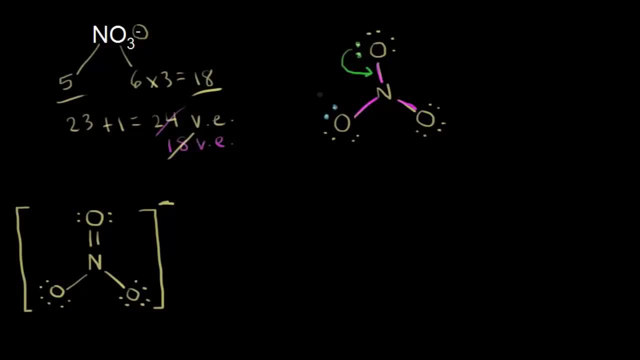 We could have taken a lone pair of electrons from the oxygen on the bottom left here. So if those electrons in blue moved in here, We could have drawn another dot structure Which would have been equally valid. right, We could have shown this oxygen on the bottom left, now bonded to this nitrogen. 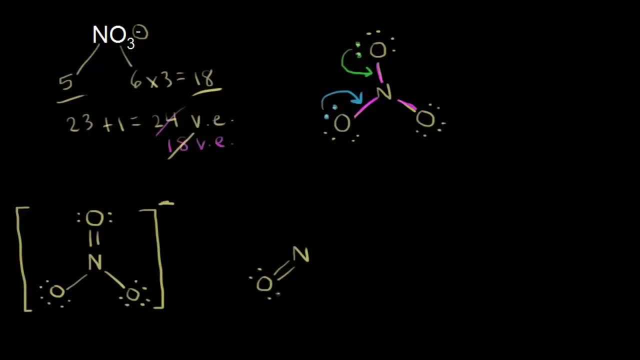 And it used to have 3 lone pairs. Now it has only 2.. And now this top oxygen is still a single bond with 3 lone pairs around it, And this bottom right oxygen is still a single bond with 3 lone pairs around it. 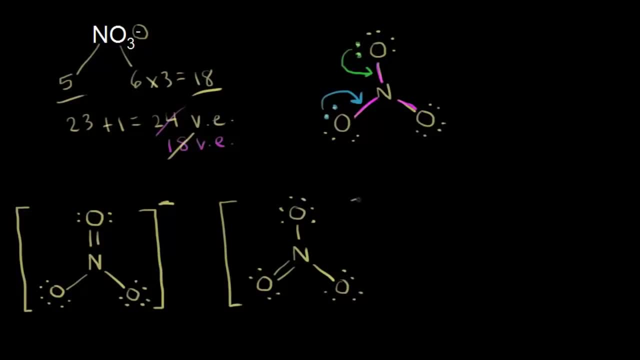 So this is a valid dot structure As well. So let's go ahead and put our brackets with a negative charge, And then, of course, We could have taken a lone pair of electrons from the oxygen on the bottom right, So I could have moved these in here to form a double bond. 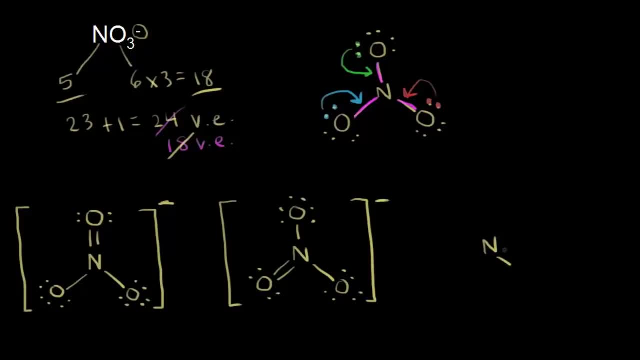 And so now we would have our nitrogen double bonded to an oxygen on the bottom right. The oxygen on the bottom right now has only 2 lone pairs of electrons. The oxygen at the top Single bond with 3 lone pairs, And then the same situation for this oxygen on the bottom left. 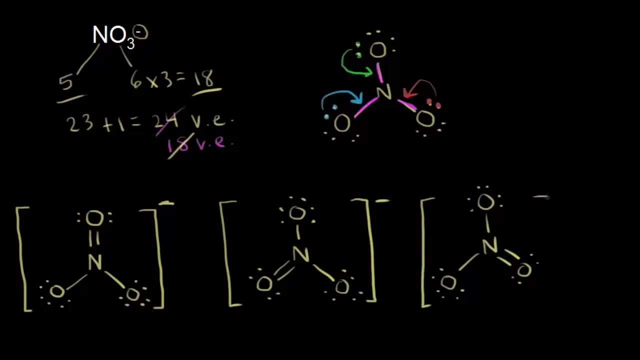 And so this is once again another possible dot structure And so these are considered to be resonance structures of each other, And the way to represent that would be this double headed resonance arrow here. And I think when students first see resonance structures The name kind of implies that in this case the ion is resonating back and forth. 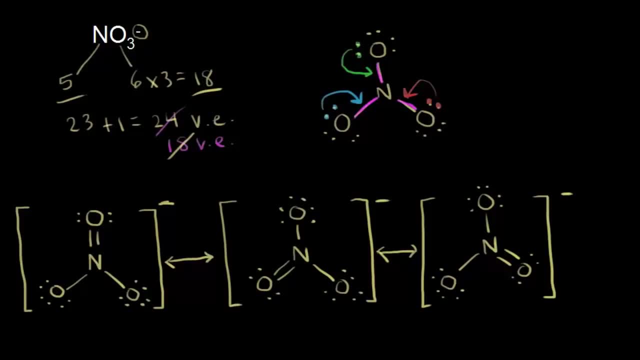 Between these 3 different possible, equally valid dot structures, And that's not quite what's going on here. Each of these dot structures is an attempt to represent the structure of the ion, But they're really not the best way of doing that. You need to think about combining these 3 dot structures in a hybrid. 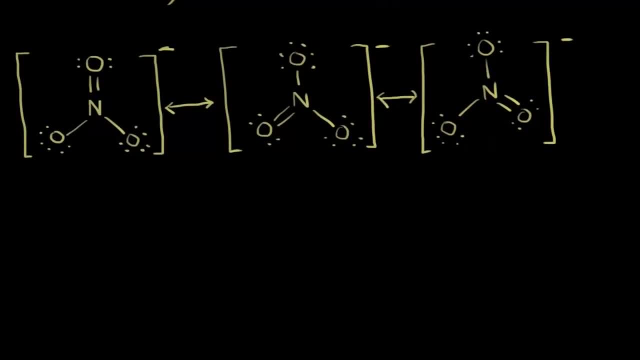 So a resonance hybrid of each other. And so let's go ahead and draw just a simple representation of a way of thinking about a resonance hybrid. So if I kind of combined all 3 of my dot structures here into one picture, Right, I had a double bond to one oxygen in each of my 3 resonance structures here. 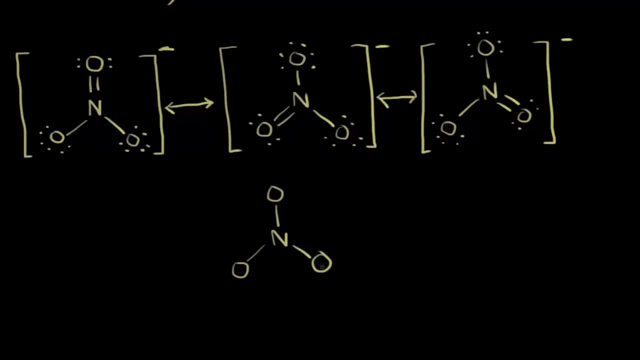 And so the top oxygen had a double bond in one of them, The bottom left in the middle one And the bottom right in the third one. So in reality, if we take a hybrid of all of those things, We can think about the electrons being delocalized or spread out among all 3 of our oxygens.